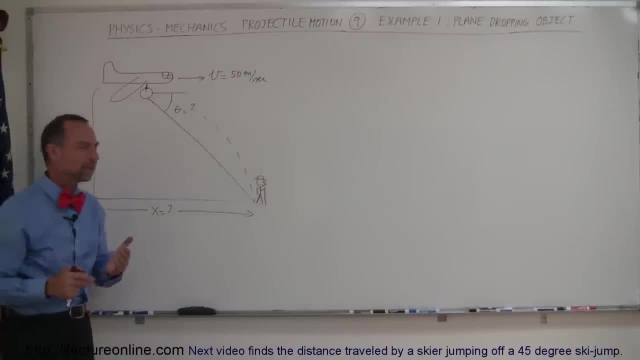 Okay, and also since, of course, a navigator typically will find that position location through an angle relative to the horizontal, we also need to find that angle. Since there is no initial velocities in an angle away from either horizontal or vertical, we don't have to find the components. 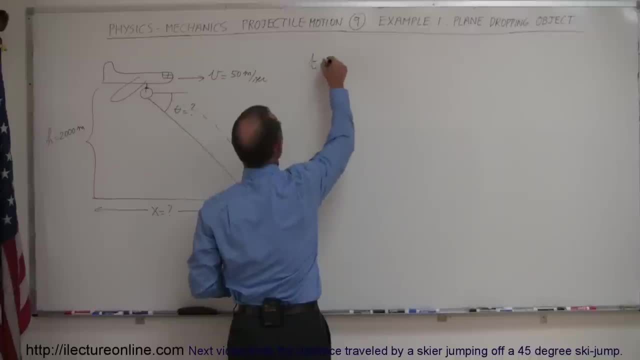 so we can go right into the approach saying time in the air is equal to question mark. Let's find the time in the air and of course the equation for that is: y equals y sub naught Plus v sub naught in the y direction. times time plus one-half gt squared. 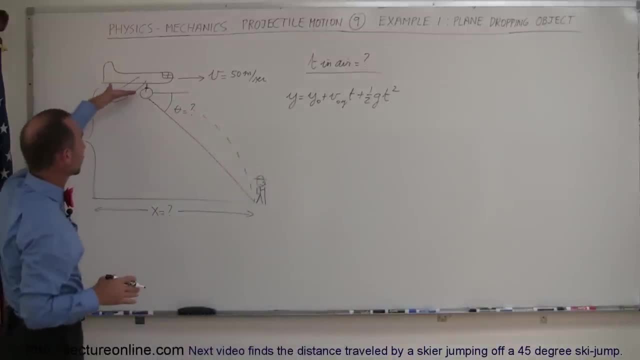 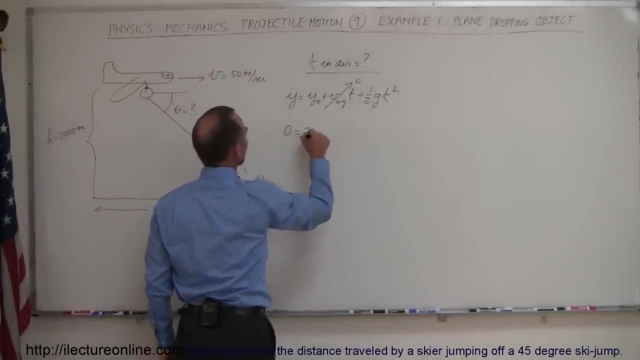 Realizing here that in this case there is no initial velocity in the y direction, because it simply dropped from something flying at a level. so this goes to zero. The final height will be zero. so we can say zero is equal to 2,000 minus 4.9t squared. 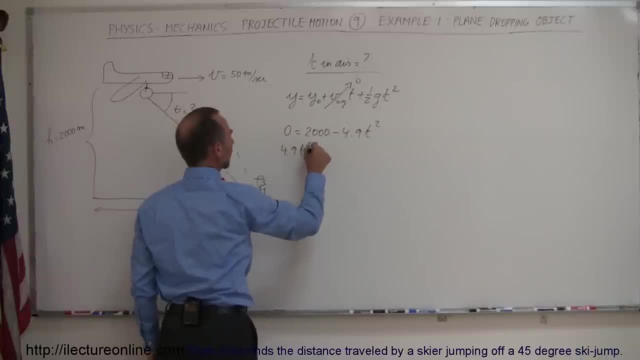 Moving that over here, we can get that as 4.9t squared equals 2,000.. Divide both sides by 4.9.. And taking the square root, we can say that t is equal to the square root of 2,000 divided by 4.9.. 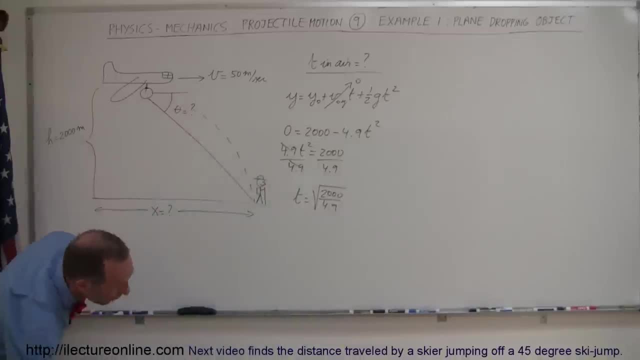 Of course, these cancel out, and let's see what that is equal to 2,000 divided by 4.9.. Take the square root and we have the time equals to 20.2 seconds. So we have time in the air. Next thing we need to do is see how far that object will fly in that amount of time. 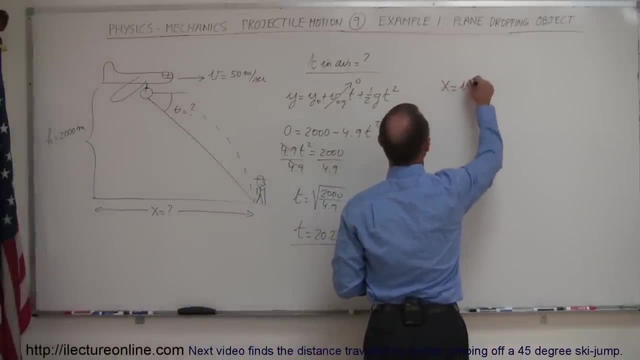 So that we can find, by using equation x Equals v, initial in the x direction times time. In this case the initial velocity of the package is the same as the initial velocity of the plane, So it will be 50 meters per second, multiplied times 20.2 seconds. 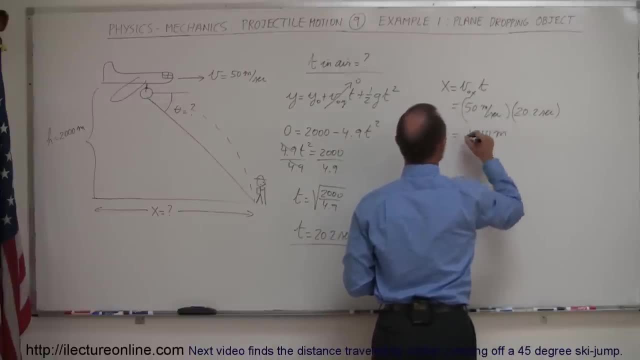 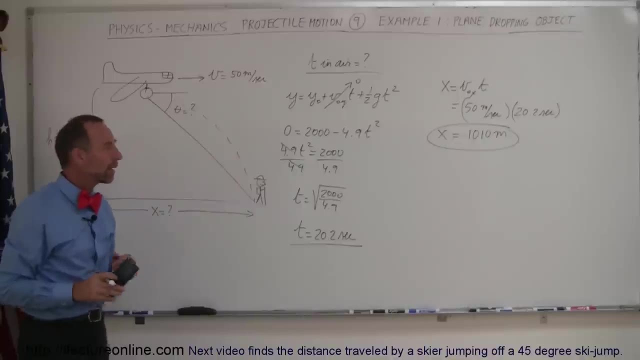 And so that would be equal to 1,010 meters. So if the plane drops the food 1,010 meters, maybe you should drop it about 1,000 meters before it gets to the Boy Scout and the package will land 10 meters behind the Boy Scout. 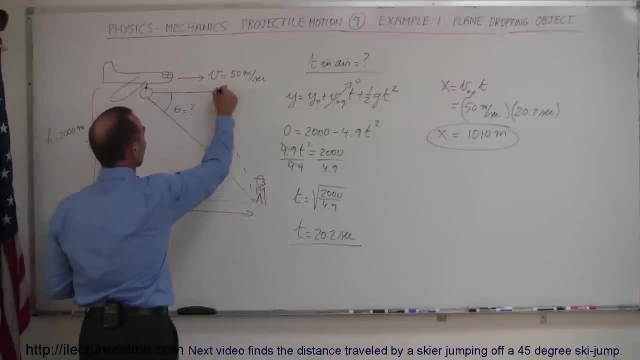 A little safer that way: 1,010 meters before it gets to the Boy Scout and the package will land 10 meters behind the Boy Scout. A little safer that way. And then, if you want to find that angle, notice that this will be a triangle.